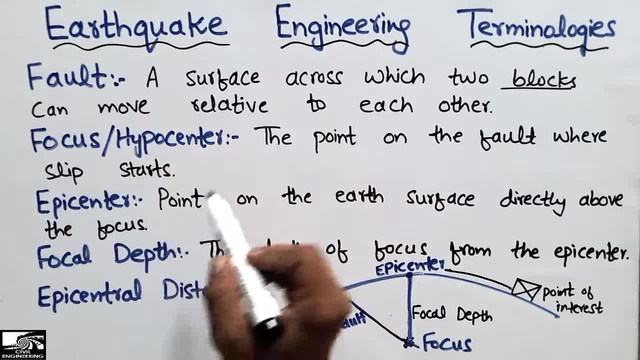 These are the synonyms of one another: Focus or Hypo Center. So it can be defined as the point on the Fault where the slip starts. So it is the point on the Fault like this: is the Fault line, for example, is the Fault You can see here. 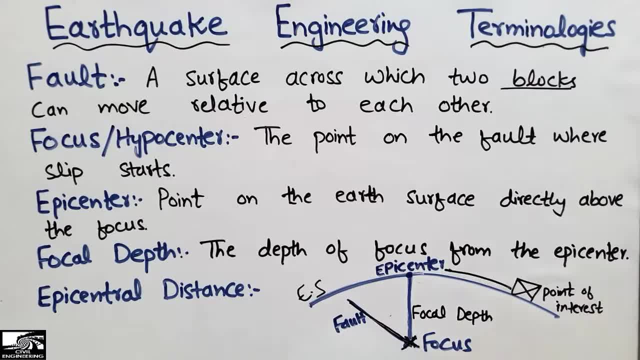 You can see here, this is the Fault, So the point on the Fault where your slip starts, where your movement of slip starts. so this point is known as the Focus or the Hypo Center. The next one is the Epi Center. Epi Center can be defined as the point on the Earth surface directly above the Focus. 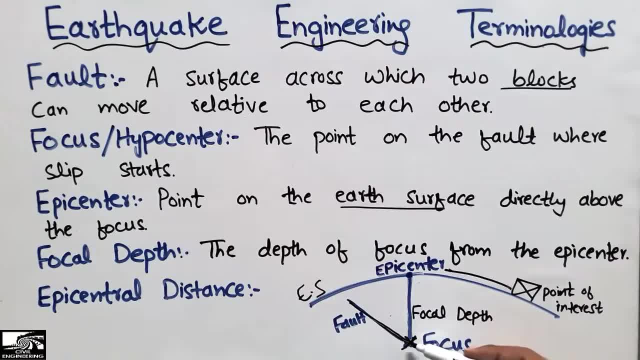 Epi Center. you can see here Epi Center. this is the point which is the above the Focus, but directly above the Focus, right, You can see here The Focus here, and above the Focus, directly on Earth's surface. this point is known as the Epi Center. 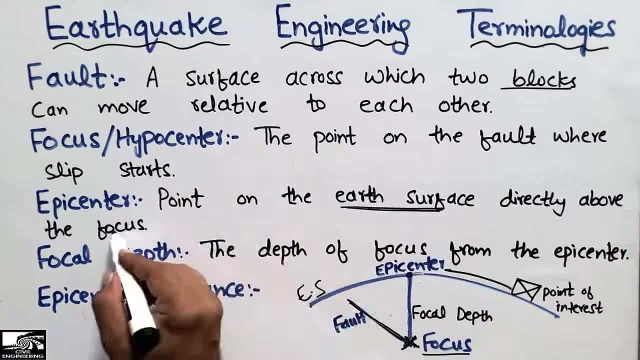 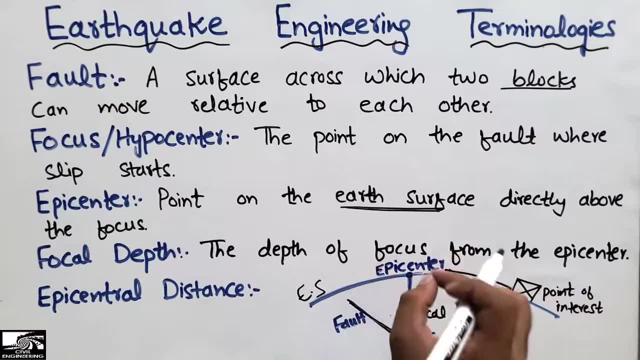 So Epi Center is the point on the Earth's surface directly above the Focus, That's, the Focus inside the Earth. So this point directly on the Earth's surface, the, this point is known as the Epi Center, which is on the Earth's surface. 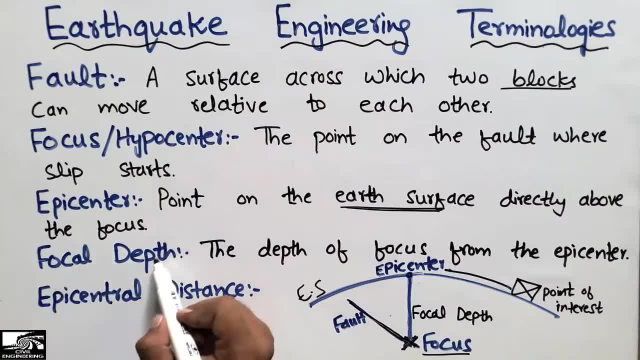 You can see here, the Epi Center is above the Focus. Now the Focal Depth. It's very simple: the Depth of the Focus from the EPICENTER up to the epicenter. this depth is known as the focal depth. the focus is below the inside of the 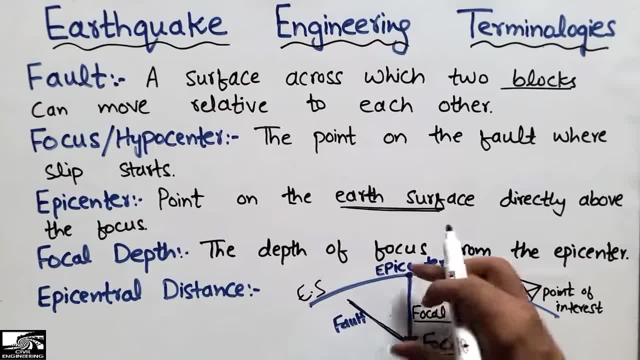 earth and the epicenter is above the earth surface directly. so this distance between these two, this is known as the focal depth. right now, what is the epicentral distance? let's suppose that we are interested, that there is some earthquake. we want to know about the earthquake information here. 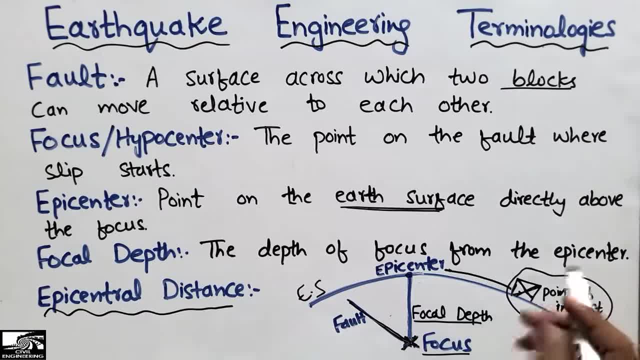 so there is some building right. so the distance from the epicenter to our point of interest, where we find the earthquake terms right. so this distance is known as the epicentral distance, the distance from the epicenter to our point of interest where we want to find the magnitude of 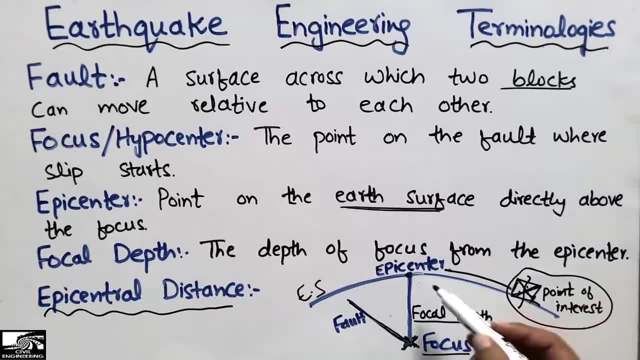 the earthquake, so are the other waves. so this distance from the epicenter to our point of interest is known as this distance. right, this distance is known as the epicentral distance. so these were the all points in the earthquake engineering terminologies. these were the basic points. right, in the coming videos i will